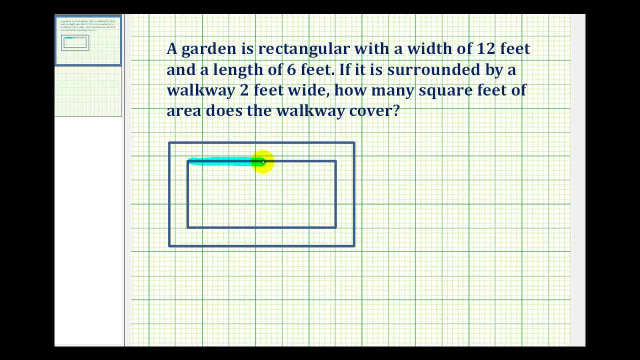 represents the garden. we could say that this length here and this length here is twelve feet, And the length of this side and this side would be six feet. The last thing we're given is that the width of the walkway is two feet. So this length here, 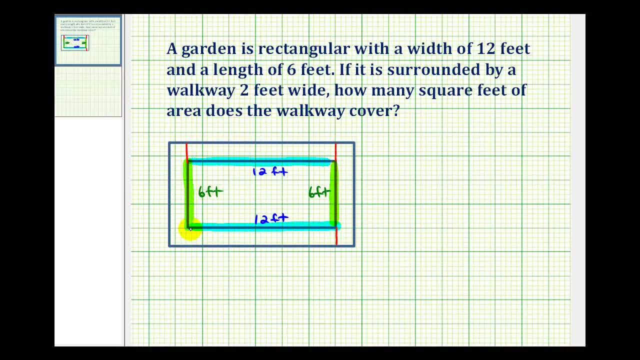 here, here and here would all be two feet And our goal is to determine the area of the entire walkway or this yellow region. So, from this sketch, to determine the area of the walkway, we need to determine the area of. 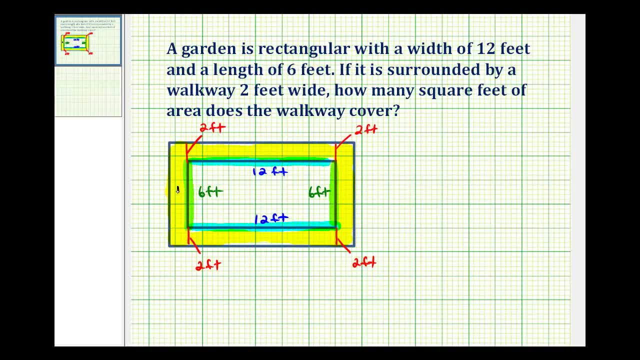 four different rectangles And we'll call this rectangle one, two, three and four, And the area formed with a rectangle is length times width. So if we look at rectangle one and rectangle two, notice they're going to have the same area. And looking at rectangle one, 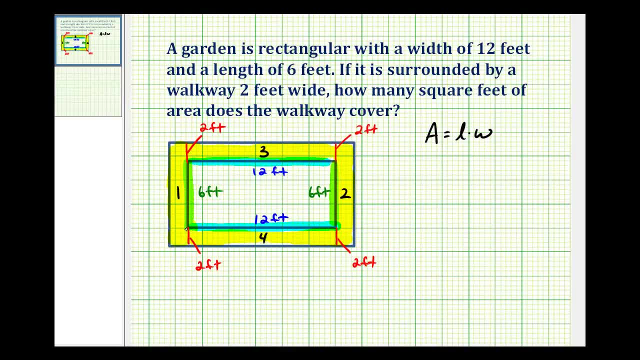 to determine the entire length of this side here, it would be six feet plus two feet plus two feet, So this entire length would be ten feet. So this rectangle has the dimensions of ten feet by two feet, which would be an area of twenty feet squared. 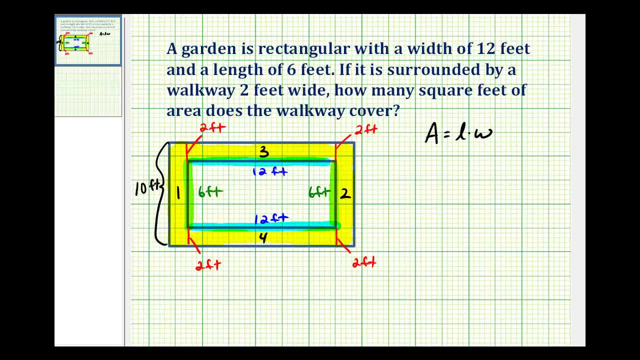 But rectangle two has the same area, So the area from rectangle one and two would be forty feet squared. Again, this is from rectangle one and two. And then for the area of rectangle three and four, looking at rectangle three, the rectangle's going to have the dimensions of twelve feet. 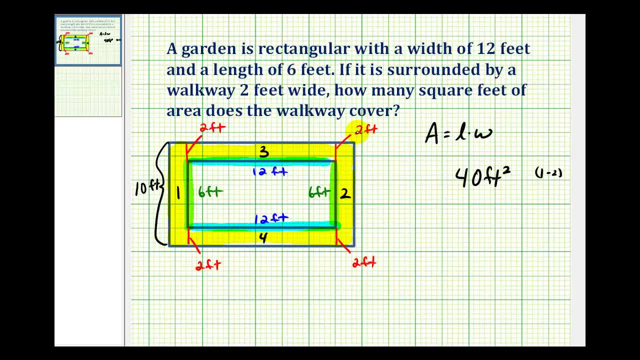 by two feet. Twelve feet times two feet would be twenty-four feet squared, But again rectangle four has the same area, giving us a total of forty-eight square feet. Again, this is from rectangle three and four, So the sum of these two areas. 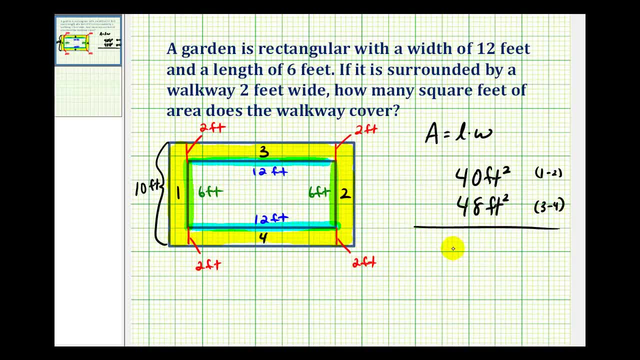 would be the area of the entire walkway, So it looks like we have eighty-eight feet squared for the area of the yellow walkway. I hope you found this helpful.